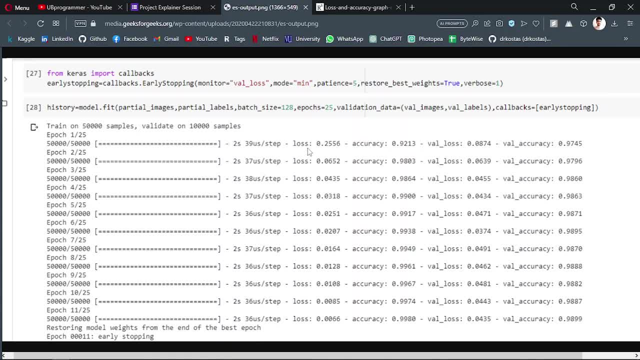 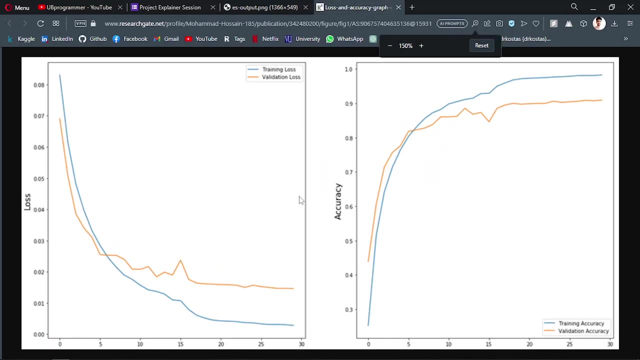 Okay, so there will be two things which you have to print when you are training. This is training happening, That means model is learning the patterns on your data and we have to report the loss and accuracy. But what this means, right? We have the graph also here. We will talk about that also. But let's see how these numbers interpret, right? 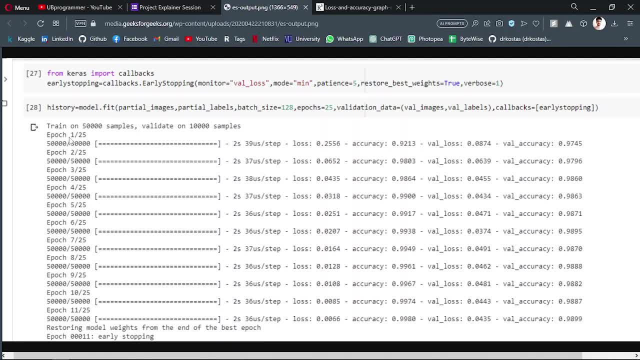 Okay, so this is epoch one. By the way, epochs just mean that your how many times your models see all of your data points. So let's say, if you are building an image classifier and you have 10,000 images in your data, then if you are choosing epoch as 10, right, 10 epochs, then it will say that the model will see those 10,000 images. 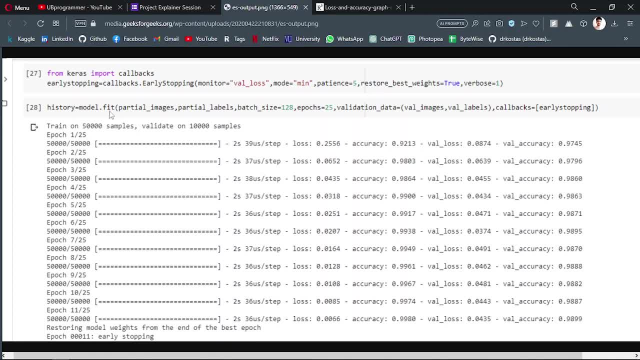 For the 10 times. Okay, so that's how it goes with the epochs. Now we know the epochs. So first epoch is happening and here are 50,000 data points. That means 50,000 images or 50,000 like any data points, right Rows of your data. Okay, so first epoch is happening. What is the loss? 0.25.. The accuracy: 0.92.. 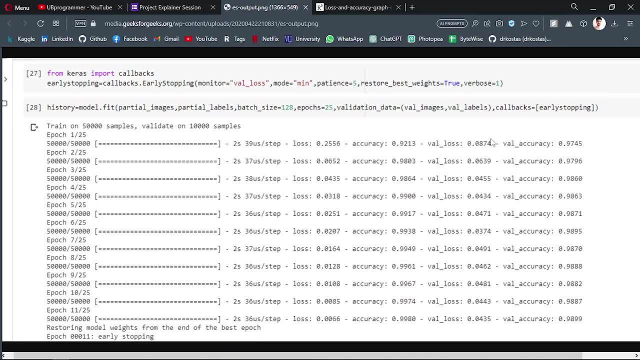 Validation loss. The loss on your testing data set is 0.08.. Validation accuracy: 0.97.. You have to be careful about these numbers. Just remember that. right Now, second epoch happening. That means model is learning and growing. right Now, what's happening? The loss is decreasing gradually: 0.06.. It happened from 0.25 to 0.06.. That big you can say decreasing. 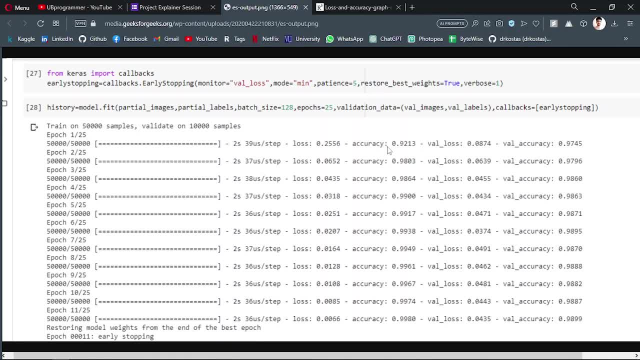 And the accuracy will be opposite from the loss. It will increase as the model learns. So from 92% it became 98%, Same with the validation loss and the validation accuracy. So that means we can conclude that loss and accuracy are totally opposite things. but loss will be higher in the beginning of the training and accuracy will be lower in the second epoch. 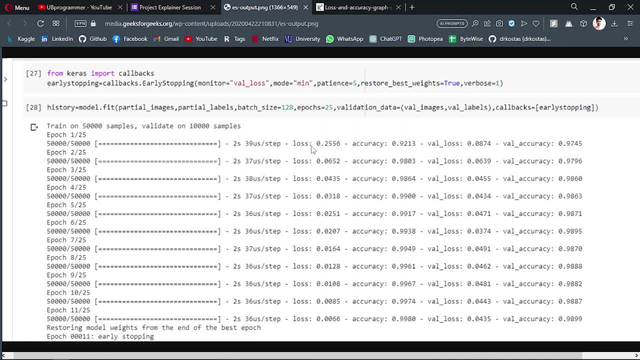 the beginning of the training. You can just note down this or just rewind the video. It may be confusing, right? And when the neural network start learning, the loss will decrease. Loss means the cost function or the error of in your prediction. It will decrease because model is understanding and learning or becoming smarter, right, With the every epoch going on And the accuracy. 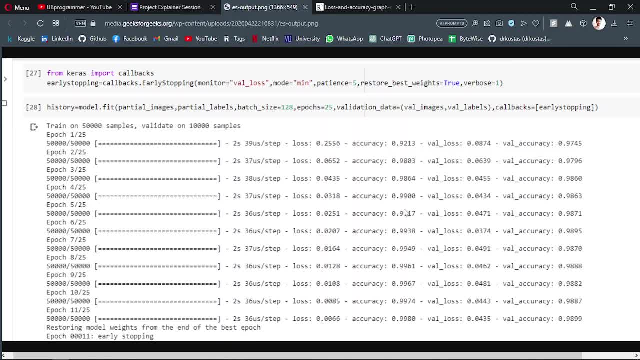 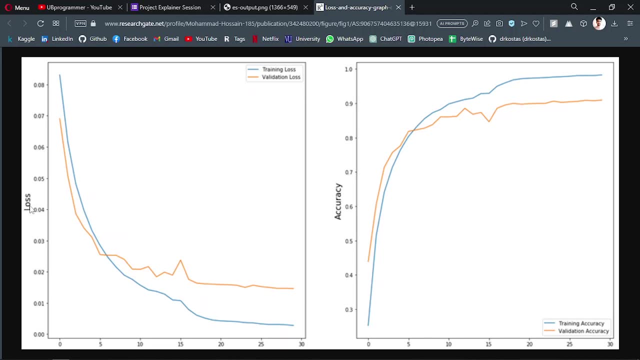 see will as, as a result, increase as the epoch will increase, right? so i hope this makes sense and now we will see it on the graph, right? so here is the loss graph. you can see the loss was quite higher in the beginning. this blue line is training loss, the loss being calculated on your training. 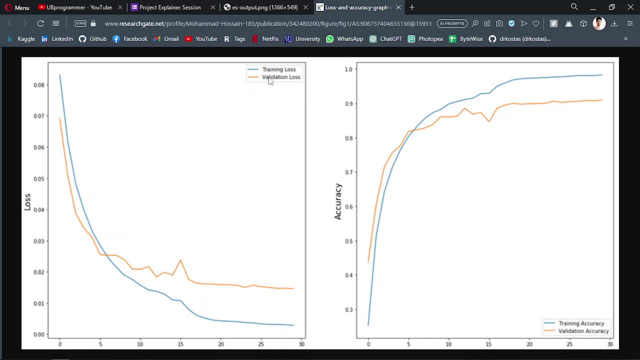 data set and the loss being calculated on your validation data set is denoted by this yellow or orange line. the loss was higher in the beginning, but it started to decrease as the model you can say: start to learn itself right. start to learn about the data and the patterns. 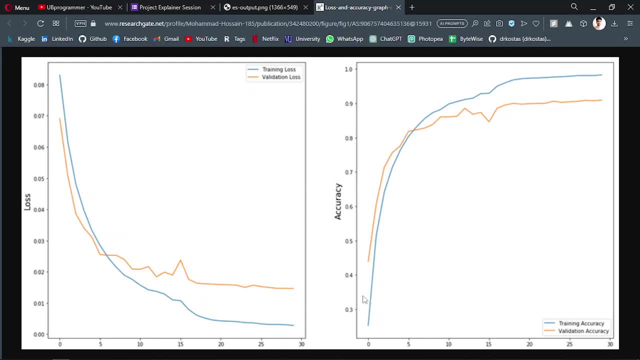 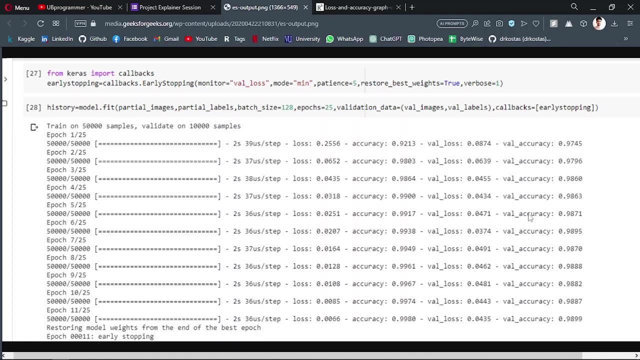 and accuracy was quite lower in the beginning but it started to increase gradually as the model start learning. so this was main interpretation of all of these numbers. so sometimes we beginners see these numbers and we just like bang our head in the world, like what all these means? so they are just numbers, but they are trying to tell you a story that model is. 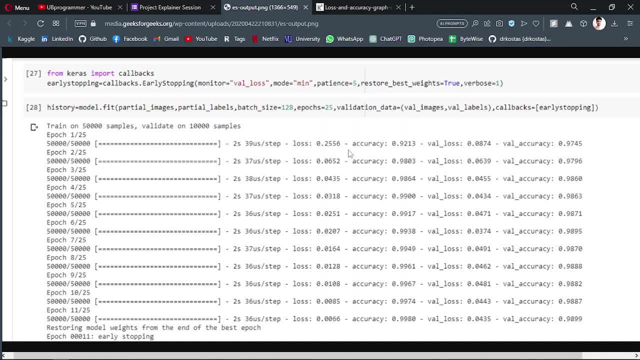 learning and you can just go on. now let's say: if the loss is not decreasing, it may be increased in. sometimes, if, if your model is not learning, if it may be a problem with your data or your approach- sometimes right. so you can just terminate that because you now understand these numbers and you can say: if the loss is increasing, then what's the? 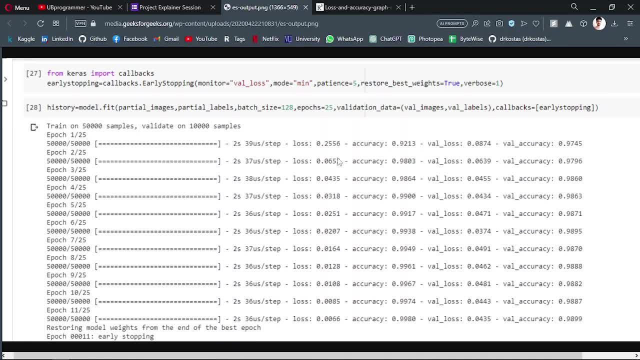 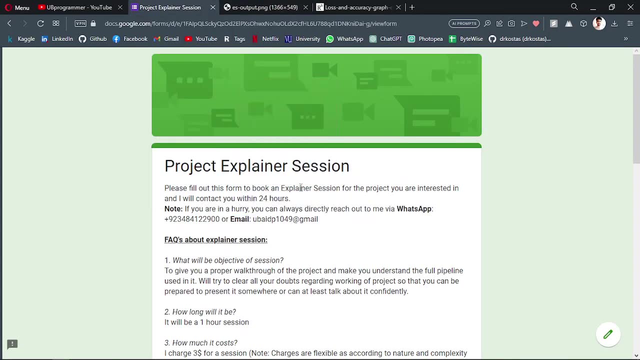 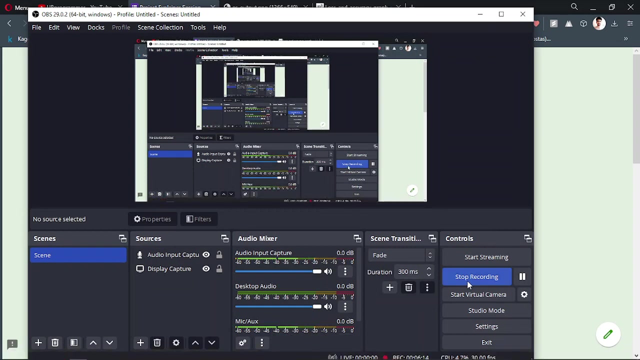 point of training further, right, so better to terminate it and start tracking your mistake in your approach, right? uh, so that's it for the video, and you can contact me on the whatsapp or mail to discuss anything about machine learning, deep learning projects or anything like that. okay, so that's it for this video. i'll meet you in the next one. 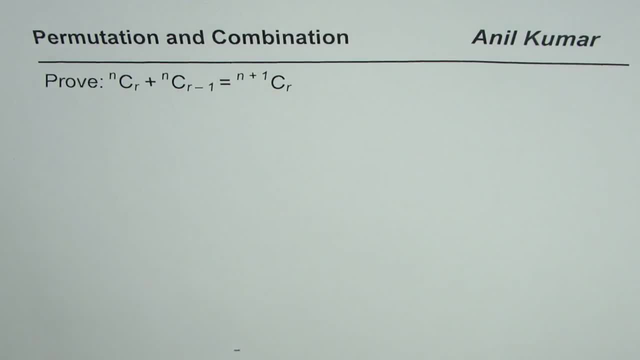 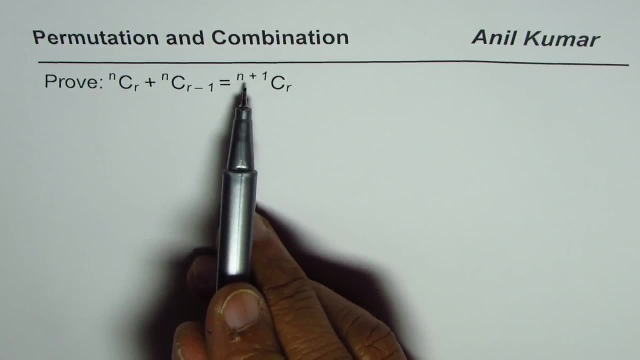 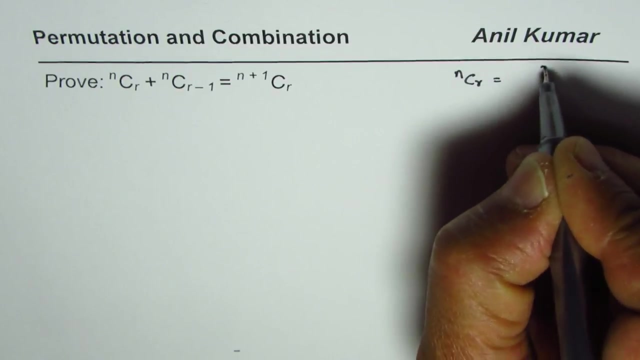 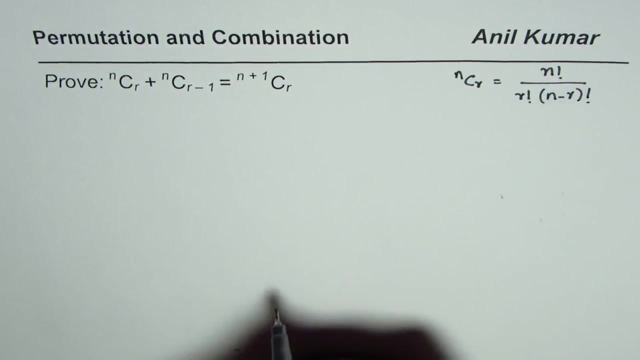 I am Anil Kumar and in this video we will prove the identity. ncr plus ncr minus 1 equals to n plus 1 cr. So we know what ncr is. ncr is n factorial divided by r factorial times. n minus r factorial. 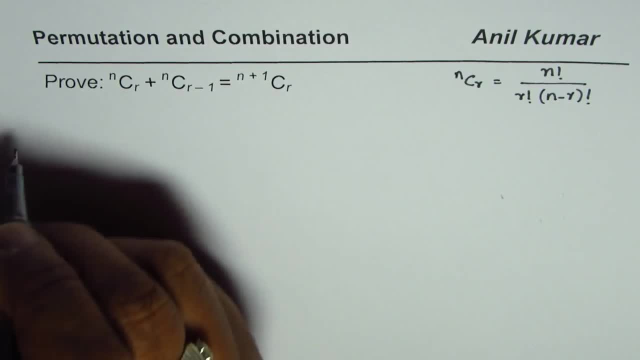 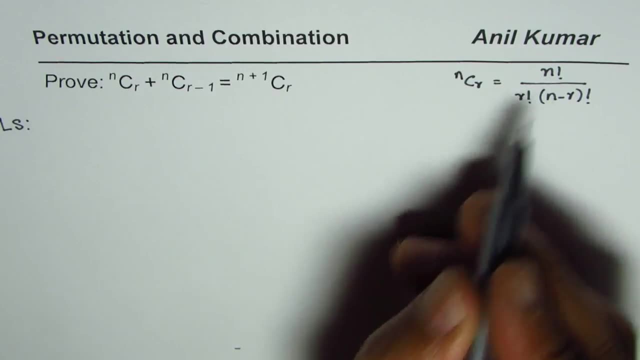 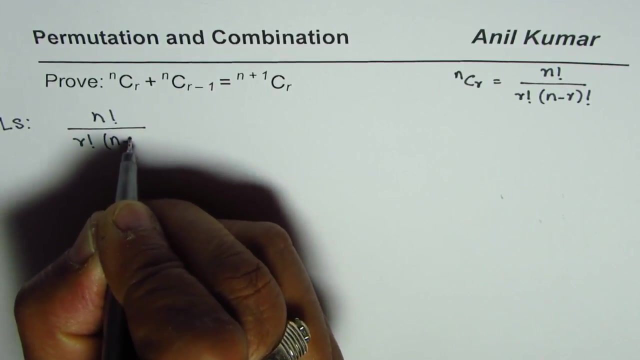 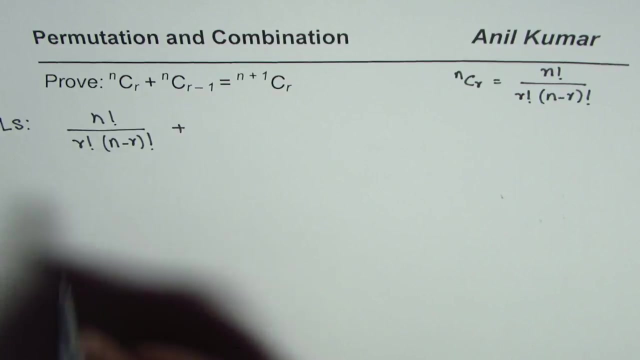 So using this formula, we will expand the left side. So let us begin with the left hand side: ncr plus ncr minus 1.. ncr could be written as n factorial divided by r factorial times, n minus r. factorial plus ncr minus 1.. So we will replace r with r minus 1.. We get n factorial. 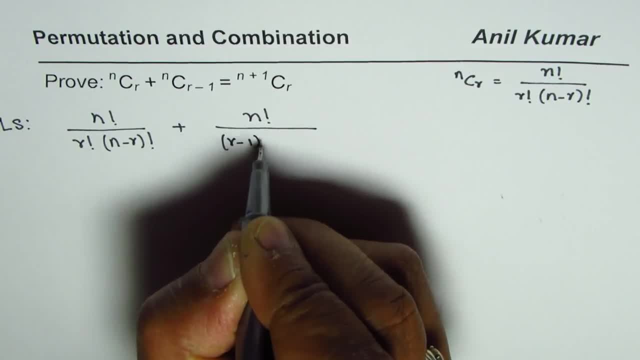 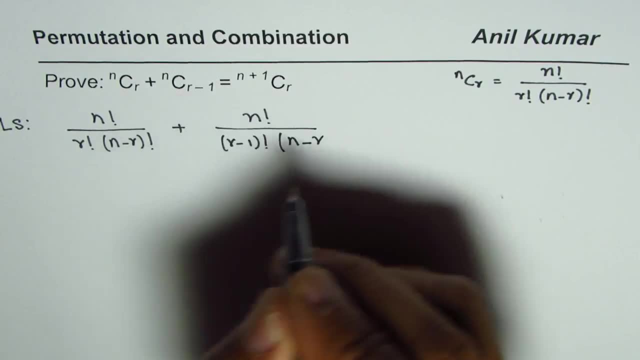 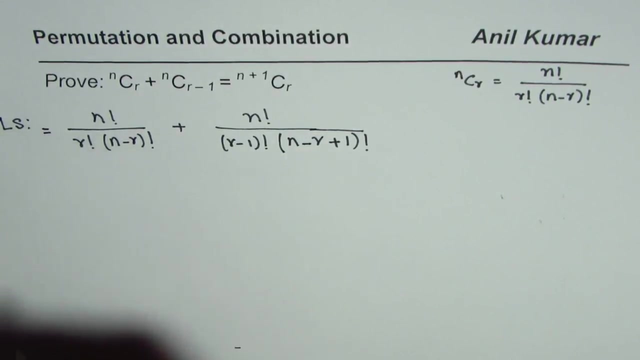 divided by r, factorial, r minus 1 factorial times n minus r and minus of minus 1 becomes plus 1, correct factorial. So that is the left side for us. So this is equal to left side. Now we have to add them. 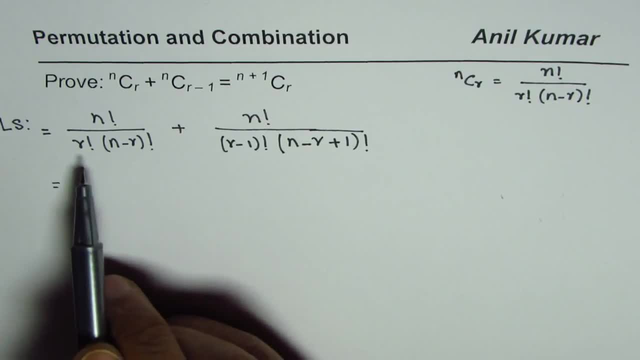 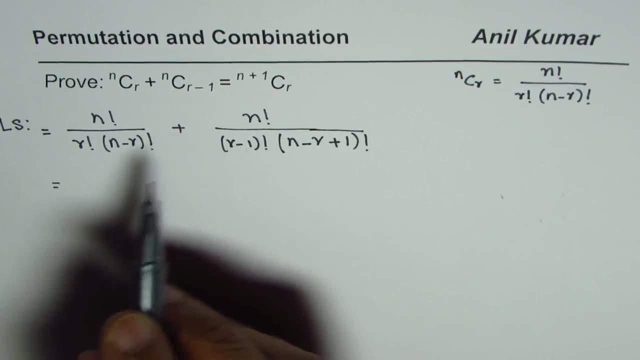 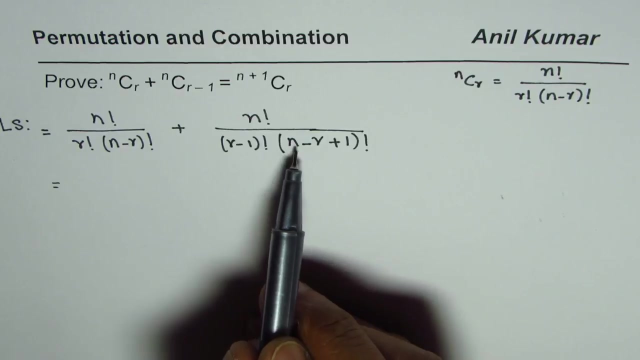 To add, we should have common denominator. Now, here we have r factorial. In this case it is r minus 1 factorial. We need to multiply this by r. right On the left side we have n minus r factorial. Here we have n plus 1 minus r factorial, Do you?